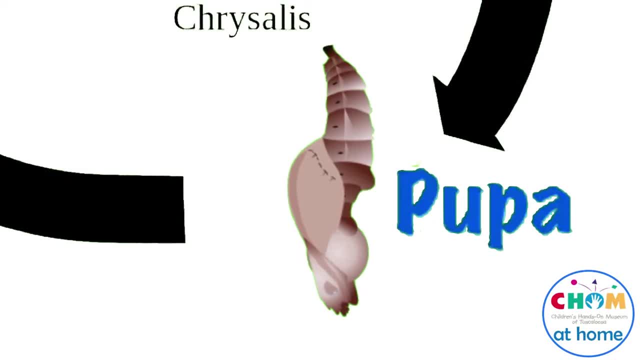 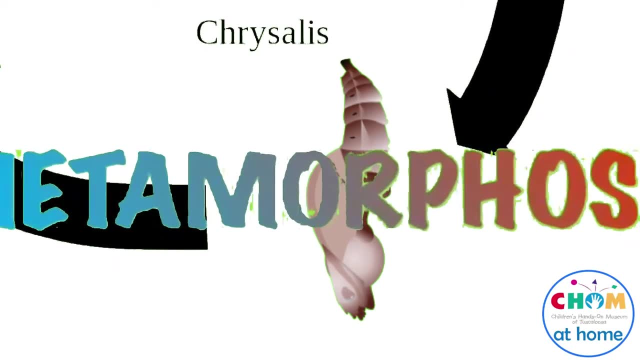 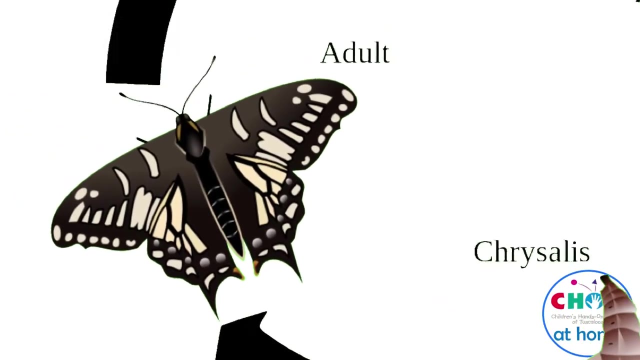 This is where the magic happens. The insect goes through something called metamorphosis. Metamorphosis is a really big word. that really just means the insect is changing For a caterpillar. this is where it forms its wings and it becomes a butterfly. After this pupa stage, the insect is 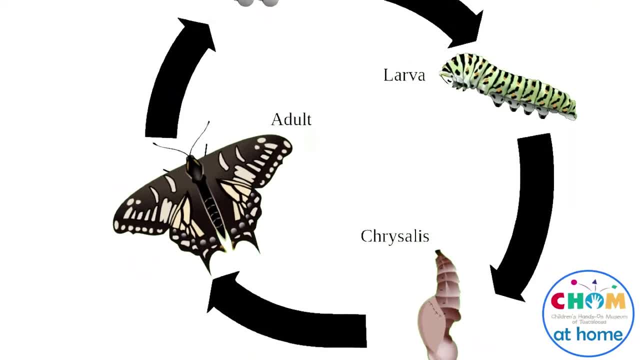 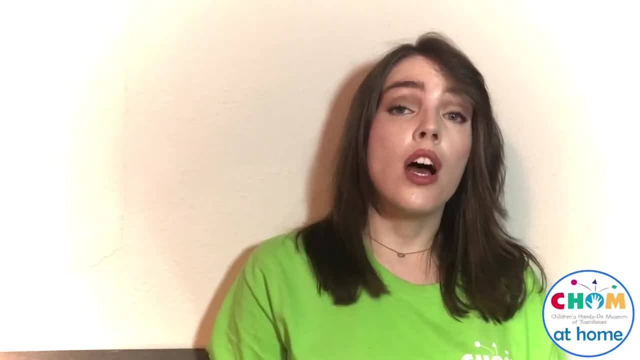 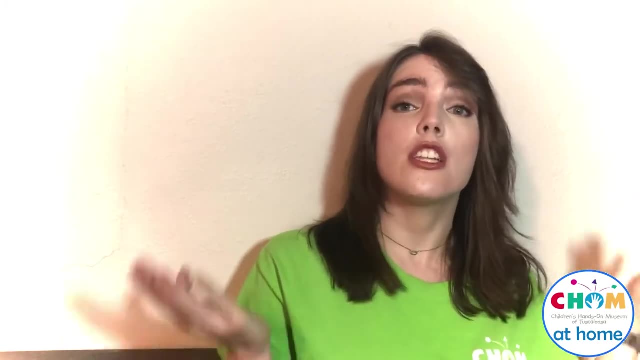 finally an adult. That adult insect will lay some eggs and then the life cycle starts all over again. The butterfly can go all the way from that egg to a caterpillar, through metamorphosis, and turn into the beautiful creature that we see outside. Some other examples of insects that go through this: 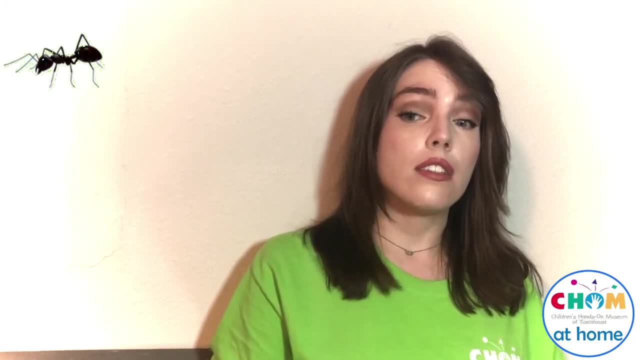 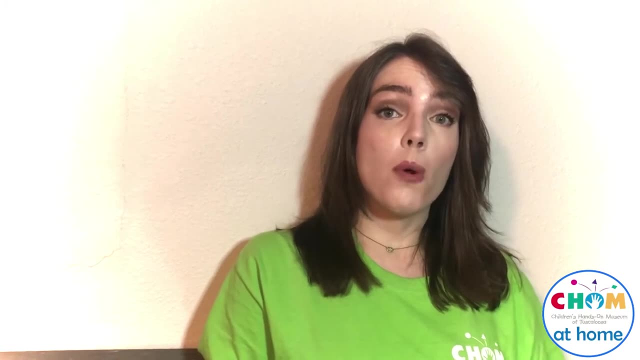 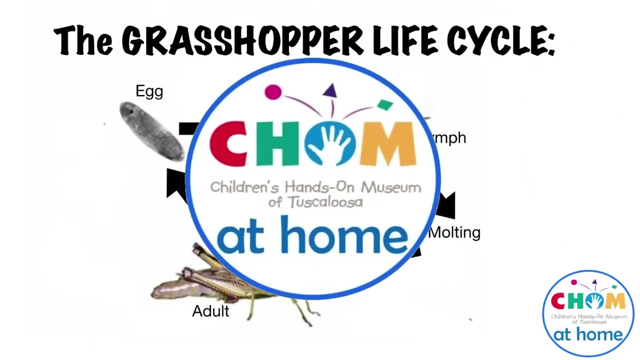 four-stage life cycle are ants, bees, moths, beetles and houseflies. But not all insects go through this four-part life cycle. Some insect life cycles only have three stages. Let's look at an example of that. This is the life cycle of a butterfly. It's a four-part life cycle. It's a. 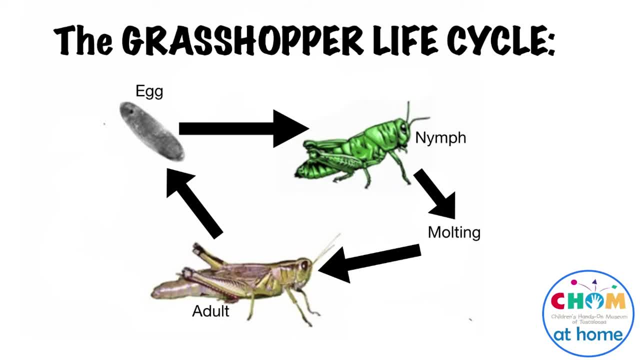 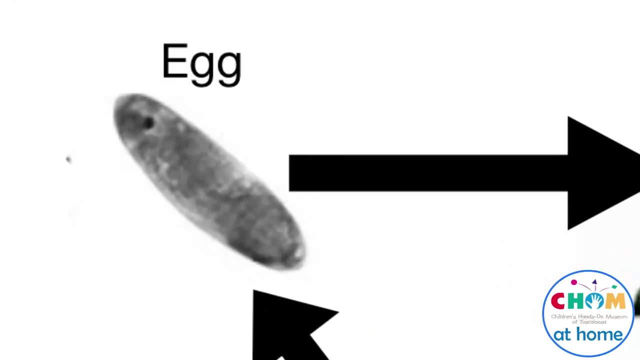 grasshopper. A grasshopper is an insect that only has three stages to its life cycle. Can you tell how it's different from the butterfly's life cycle? Well, just like the butterfly, a grasshopper begins as an egg. After that egg hatches, it's into a stage of its life cycle called a nymph. 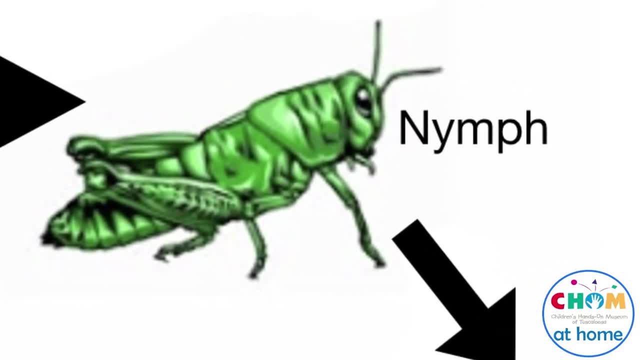 The nymph will look almost identical to the adult insect in this type of life cycle. Except, the nymph insect will not have any wings. It is not fully developed yet Once one of these insects with a three-stage life cycle like a grasshopper, is about to become an adult. 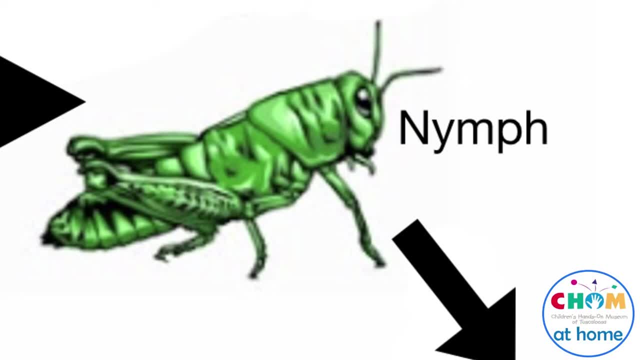 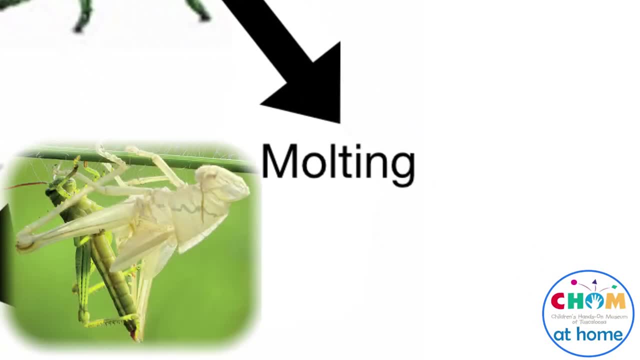 it does not have to go through any metamorphosis like the butterfly did. It just goes through something called molting. This is where it sheds its exoskeleton or kind of its outer shell, and then it's a fully grown adult. 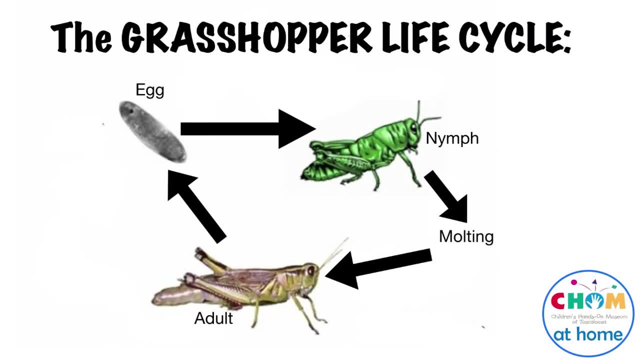 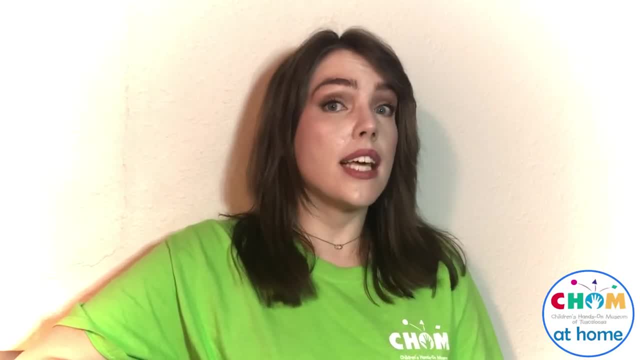 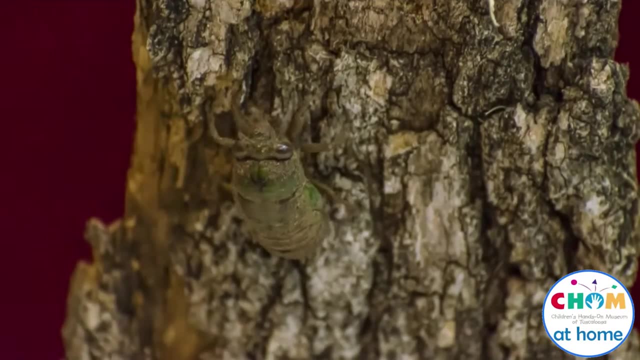 This is where the life cycle starts all over again. Another insect that goes through a three-stage life cycle is a cicada. A cicada's life cycle is pretty unique compared to other insects. This video shows a cicada molting. Now a cicada's life cycle is very, very similar. to a grasshopper, where it molts to become its adult form with its wings. What's different about the cicada, though, compared to other insects, is that its nymph stage, where it doesn't have any wings, actually lasts for up to 17 years. During all that long time,